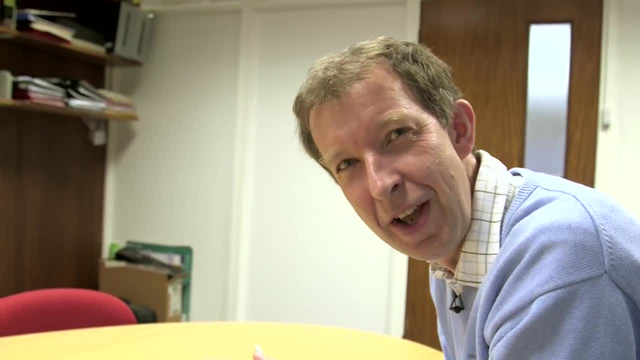 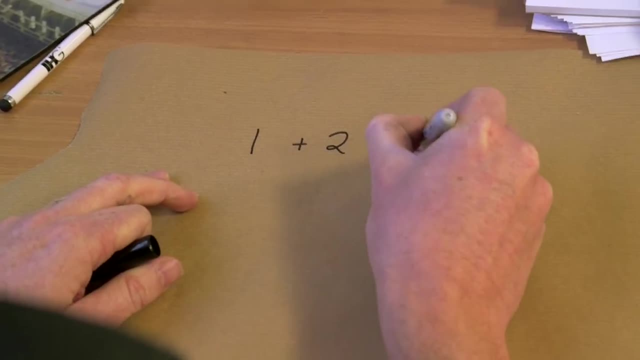 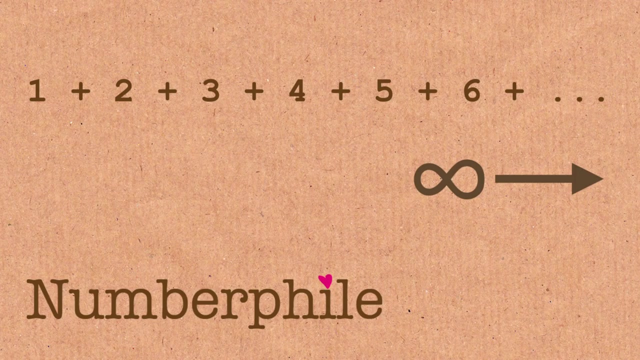 I'm going to give you an astounding result, Astounding, An astounding result. So I'm just going to write down a little sum and we're just going to see what answer it gives: 1, plus 2, plus 3, plus 4, plus da-da-da-da-da-da, and I include all the natural numbers, so all the way up to infinity. 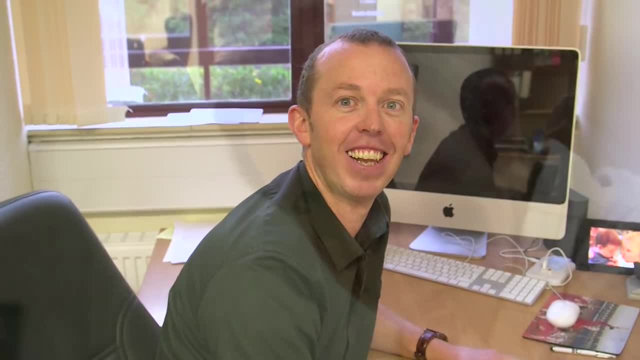 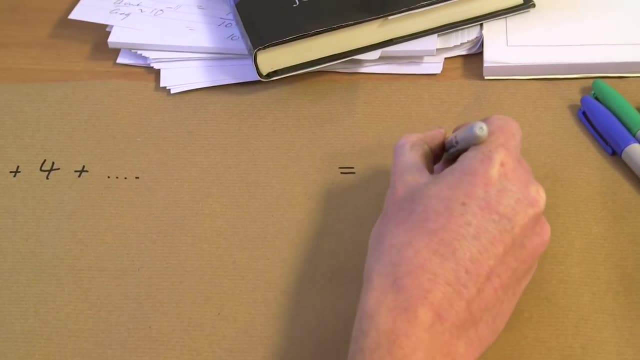 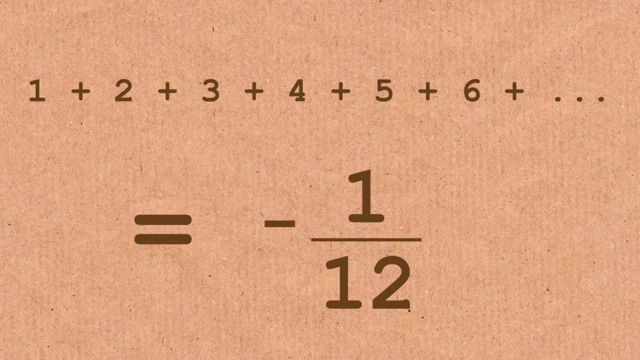 So what do you reckon? the answer to this is Brady. Well, I would say it would tend towards infinity. Yeah, that makes sense, doesn't it? The answer to this sum is remarkably minus a twelfth. It's amazing, I mean. I first saw this result when I started learning a bit of string theory. 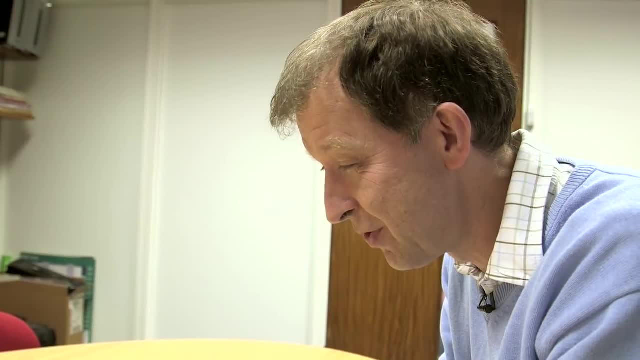 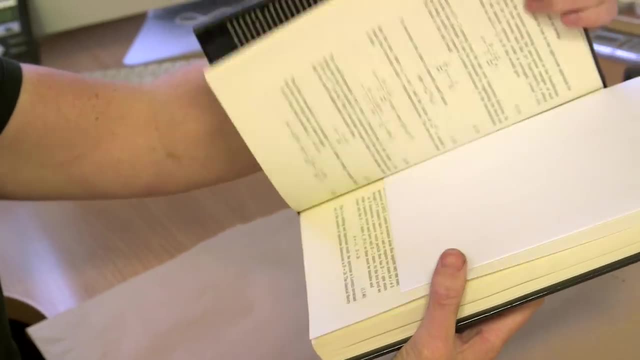 And what's even more bizarre is that this result is used in many areas of physics. This is a very well-known string theory textbook by Joe Polczynski, As you can see quite early on page 22,. we have this statement here, which is that the sum of all 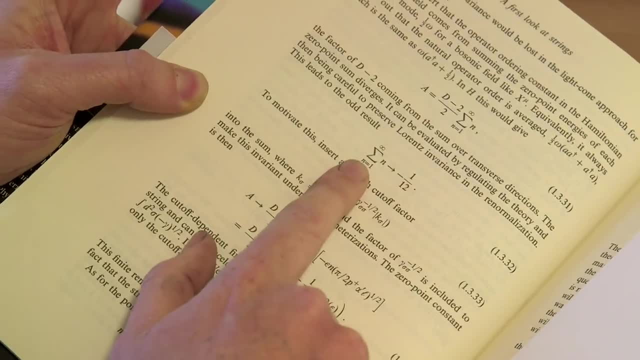 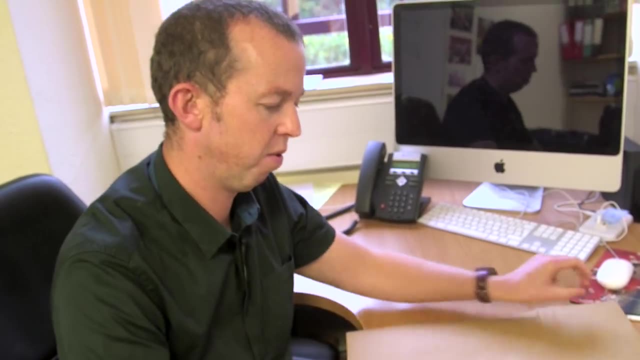 this is basically saying the sum of all the integers, Or the natural numbers all the way up to infinity, is minus a twelfth. All right, so we're going to prove now, without getting our knickers in a twist with Riemann, Zeta functions. 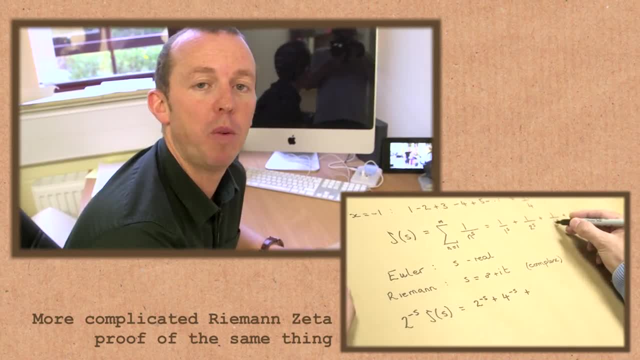 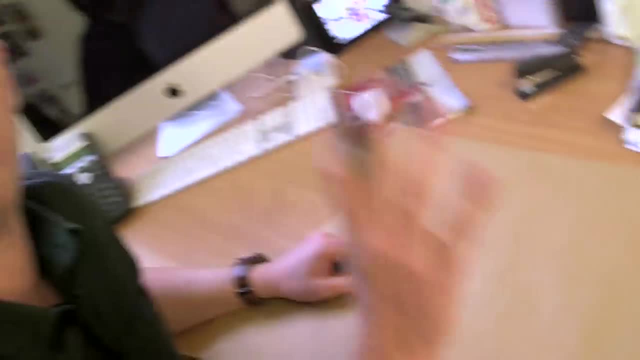 we're going to prove in quite a simple way why the sum of all the natural numbers is indeed minus a twelfth. So to do that, we're going to do this in a number of steps. We're going to look at a few different sums. 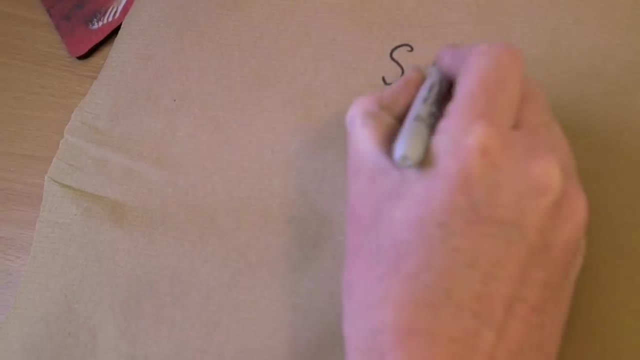 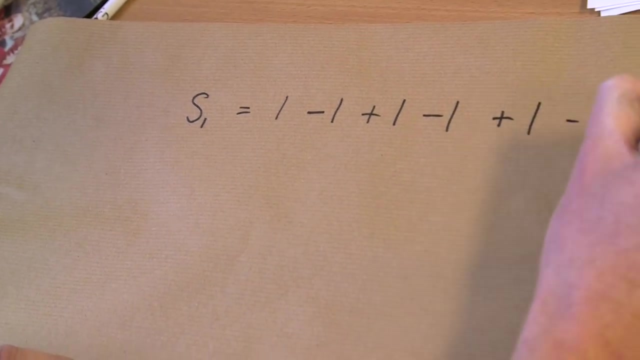 The first sum that I want to look at. I'm going to call it S1.. And it's 1, minus 1, plus 1, minus 1.. plus 1, minus 1, and so on. That's the first sum I want to look at in principle. 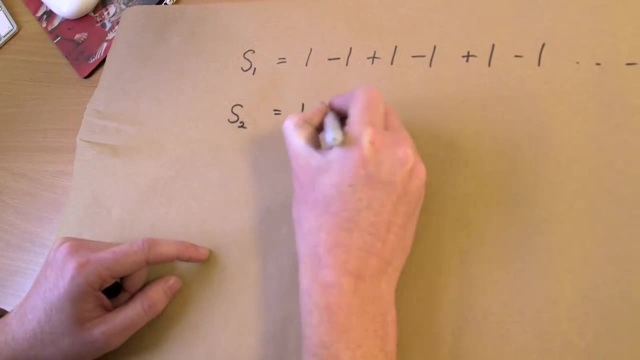 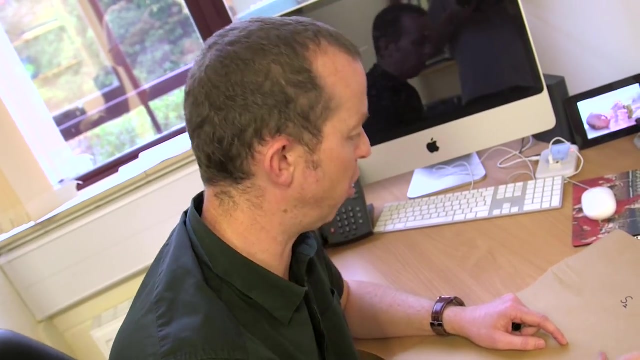 The second sum I'm going to look at is 1, minus 2, plus 3, minus 4, and so on. Carry on in that process all the way up, And the third one is of course going to be one that 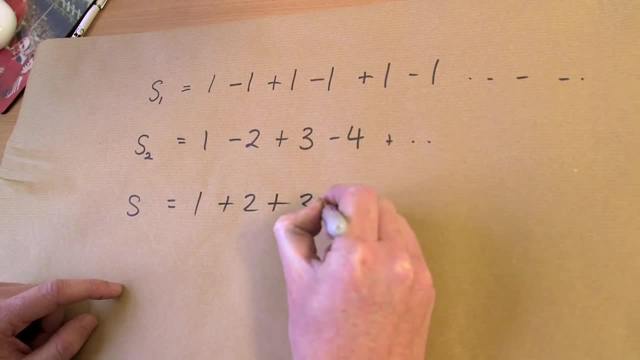 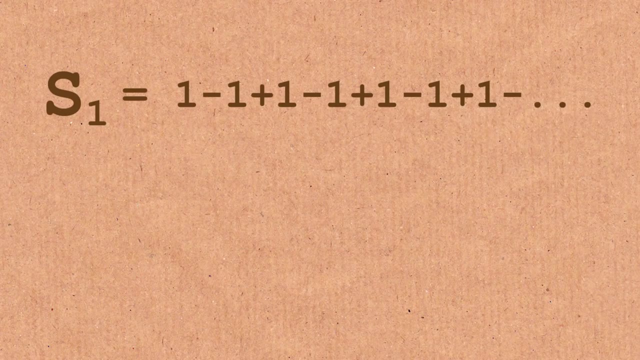 we're really interested in, which is 1, plus 2, plus 3, plus 4, and so on. So we're going to evaluate all these three different sums Now. the first one is really easy to evaluate. We need to attach a number. 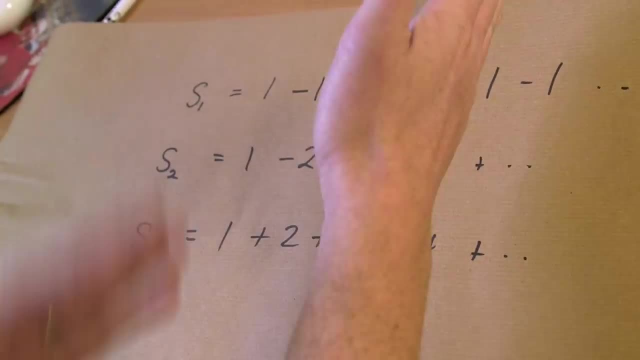 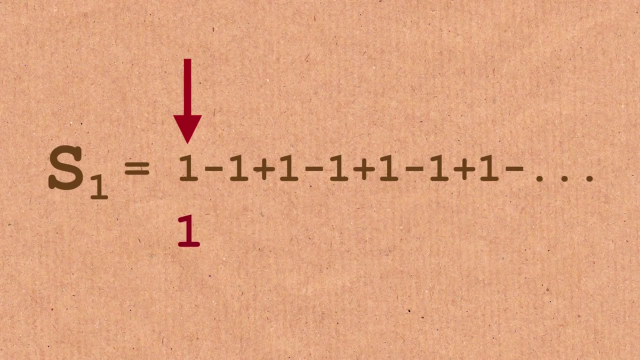 Now, clearly, what is the answer to this? Now, you stop this at any point. OK, If you stop it at an odd point, you're going to get the answer 1. If you stop it at an even point, you'll get the answer. 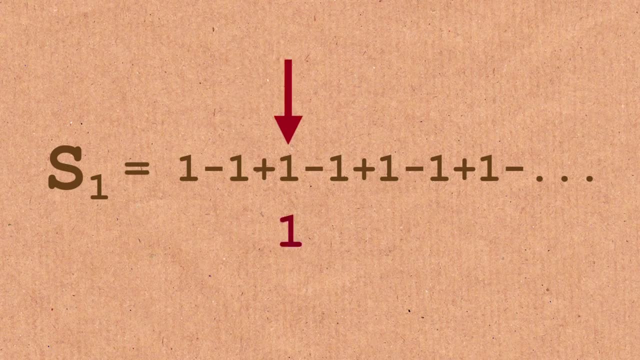 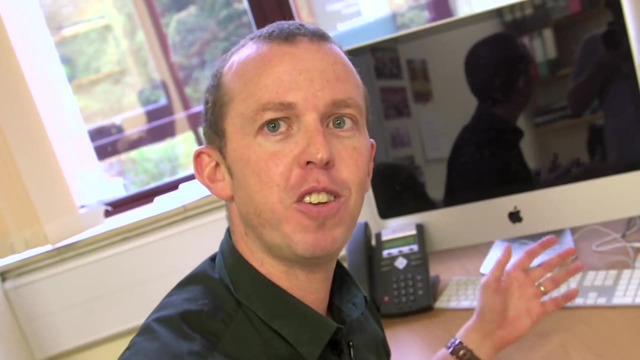 0,. clearly That's obvious, right? So what number are we going to attach to this infinite sum? Do we stop at an odd or an even point? We don't know. So we take the average of the two, So the answer's 1.5.. 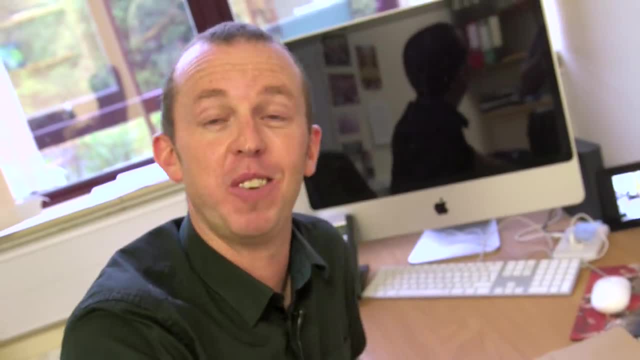 There are other ways to prove that this sum is 1.5,, by the way, which we can do If you want. No, no, there'll be a link there, because we've done it before. OK, good, So you'll see the link there. 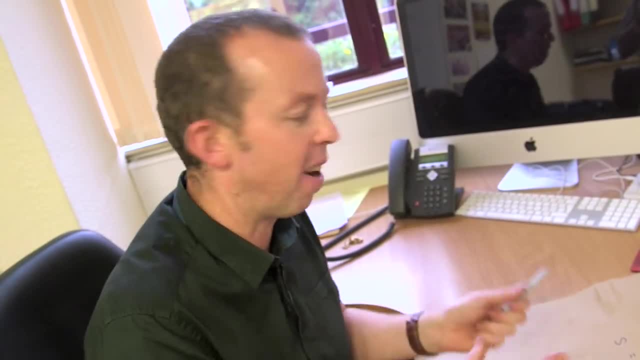 OK, so this is 1.5.. But I think, intuitively, that's the easiest way to say that you either get 0 or 1, and therefore you just take the average. So this is the natural number to attach to this sum. 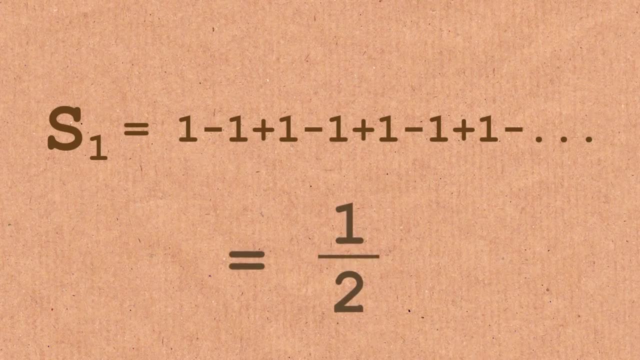 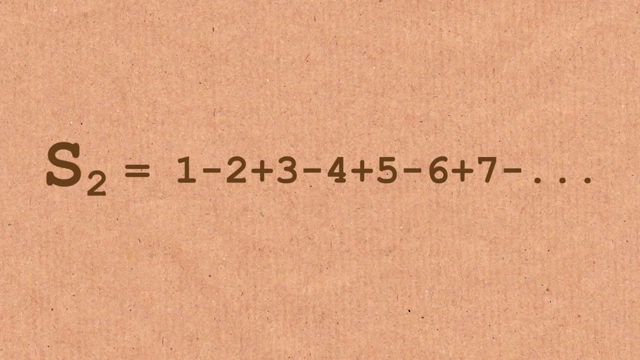 But once we know this, we're laughing. OK, Because from this we can achieve everything that we want to achieve. The next step is to find out what this sum is. So what I'm going to do is I'm going to take two copies of 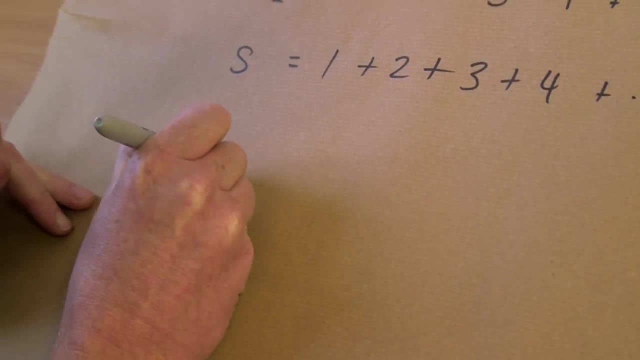 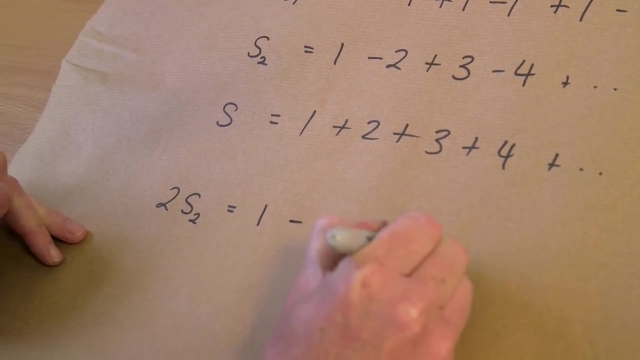 this S2, OK, So I'm going to add it to it. So 2 times S2 is equal to well, let me just write it out. So I'm going to write it out twice: 1 minus 2 plus 3 minus 4, diddle in it, and so on. 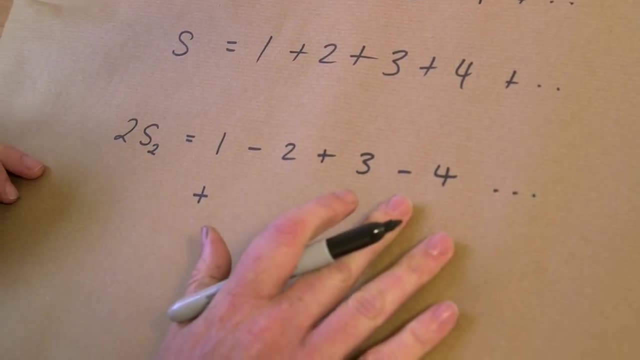 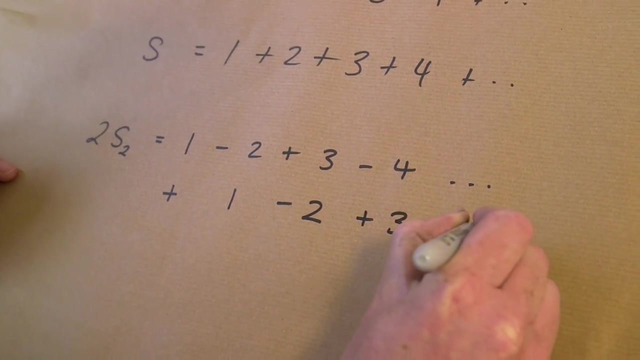 And then I'm going to add to it itself, But I'm going to shift it along a little bit, So that's plus 1 minus 2, plus 3 minus 4, and so on. OK, I've just taken two copies and added them together. 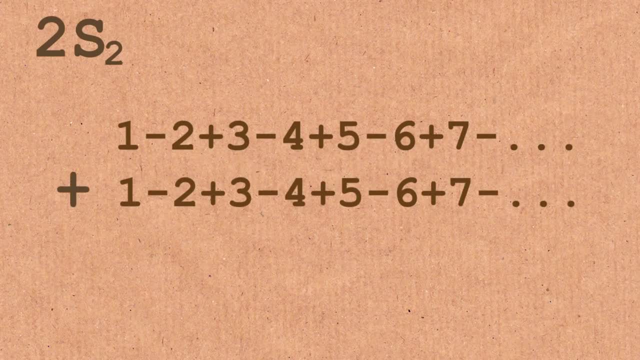 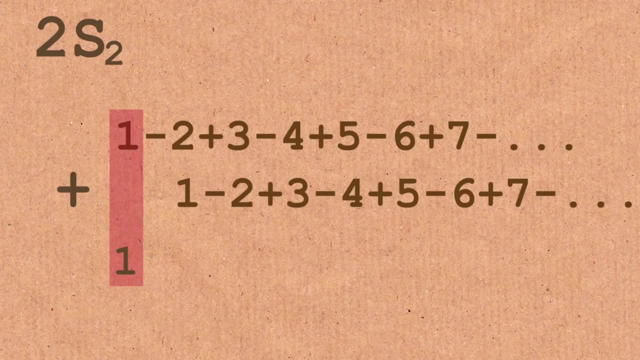 But I've done it in a particularly nice way And I just pushed this one along slightly on the bottom. So now you see what you get. You take this one and this, this and this, and I get 1.. So 1 plus nothing is 1.. 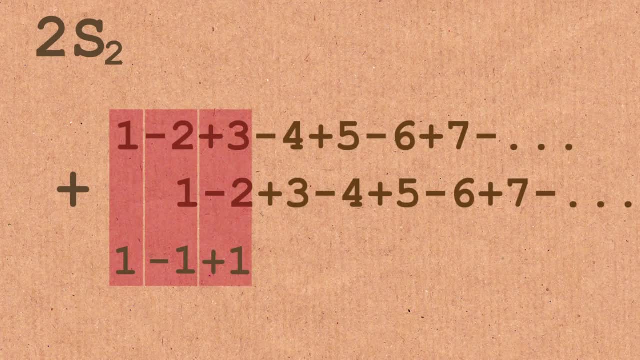 Minus 2 plus 1 is minus 1.. 3 minus 2 is 1.. Minus 4 plus 3 is minus 1, diddle, diddle, diddle and so on, and I'm going to keep getting this pattern. 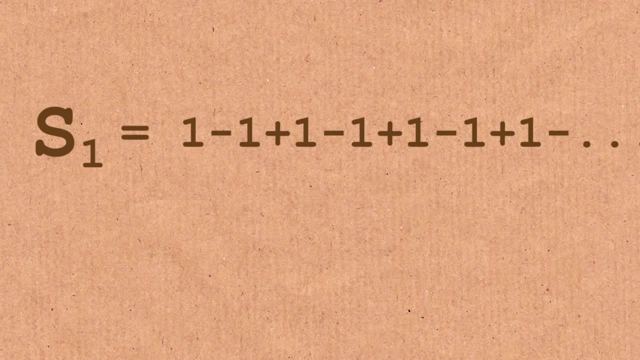 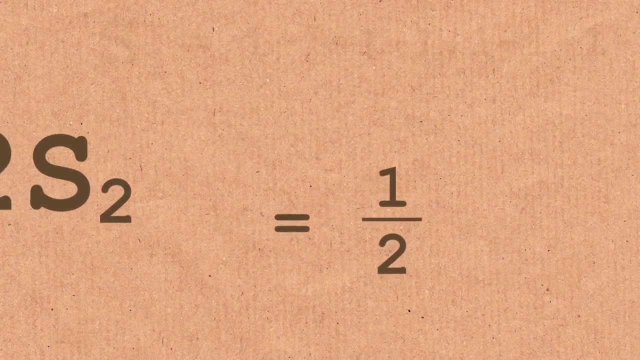 So hang on a minute. I've just got back to the sum that I started, with, which I know the answer to so half, OK. So therefore I know this sum now, because I just divide through by this 2, and I get a quarter. 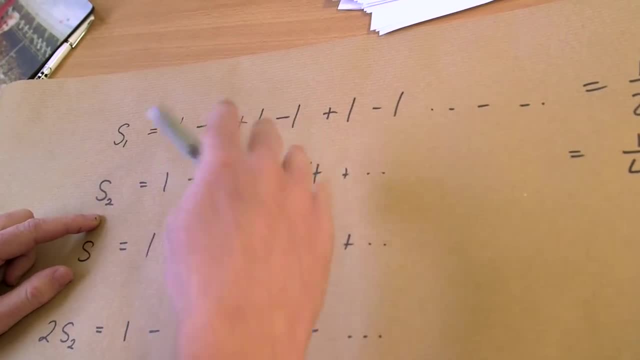 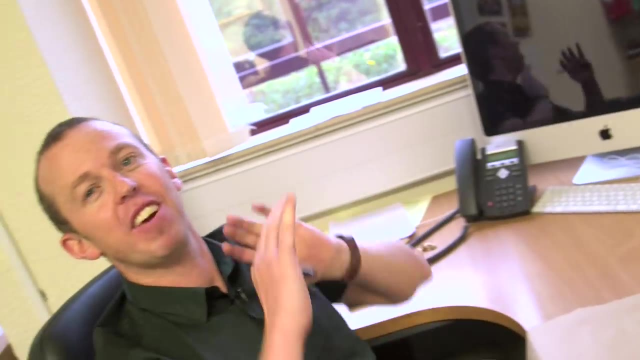 So now I know that this sum, this second sum with some where the signs alternate- is actually equal to a quarter. So this is my second remarkable result. Now I have everything I need to prove this crazy, minus a 12 thing, right. 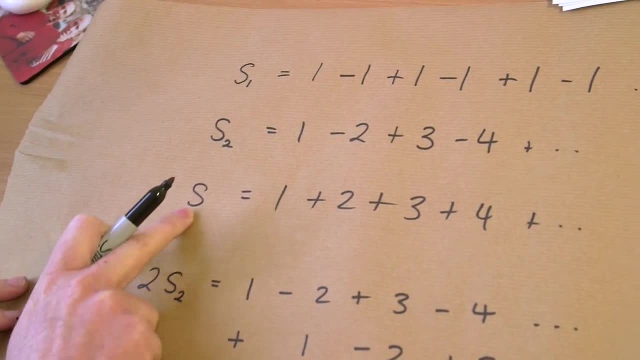 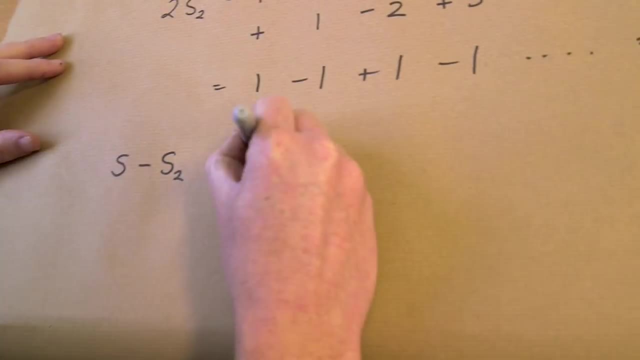 OK, so let's do it. I'm going to take this one and I'm going to subtract this one. OK, so I'm going to subtract s2 from s. Let's write them out again. OK, so I'm going to write out s first, which is 1 plus 2. 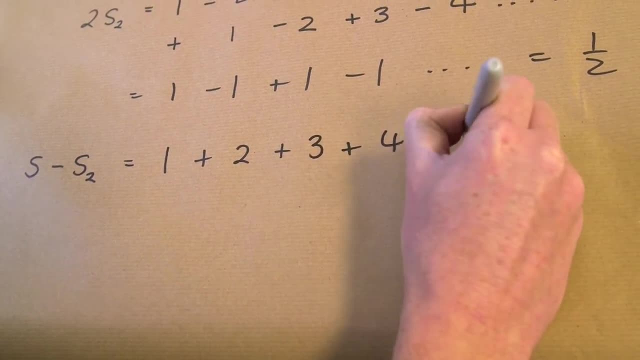 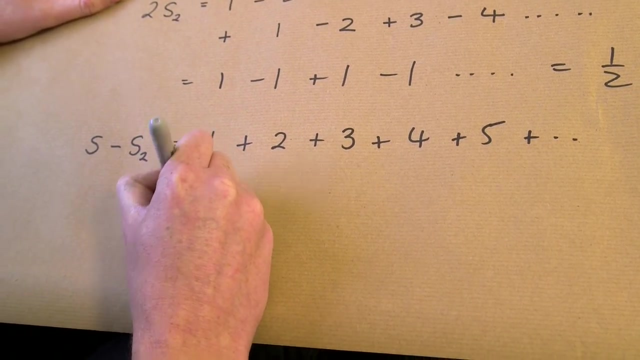 plus 3.. Plus 4,, plus 5, and so on. OK, And I'm going to subtract s2.. So that's minus. OK, and let me just put a bracket in now, because I'm going to minus all of this. 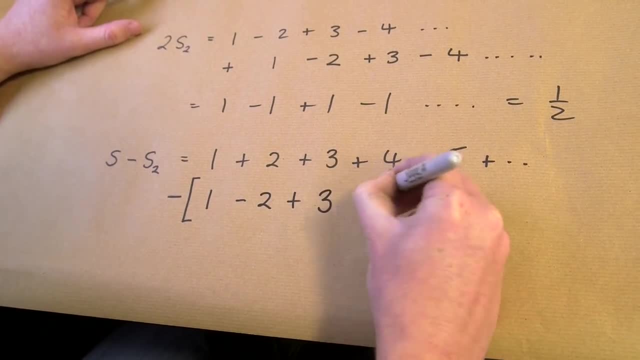 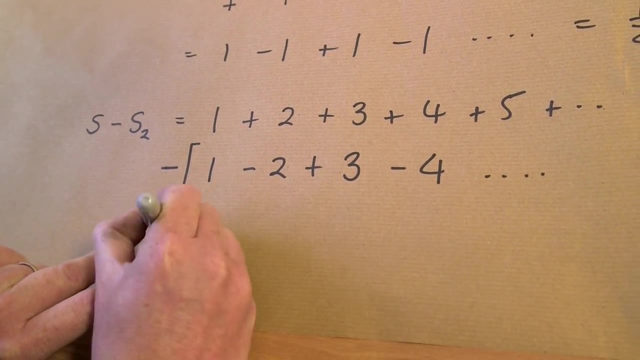 1 minus 2 plus 3 minus 4, and so on. OK, OK, 1 minus 1.. What's that? 0.. 0,? yeah, exactly, So I get nothing from that bit. 2 minus minus 2 is 4.. 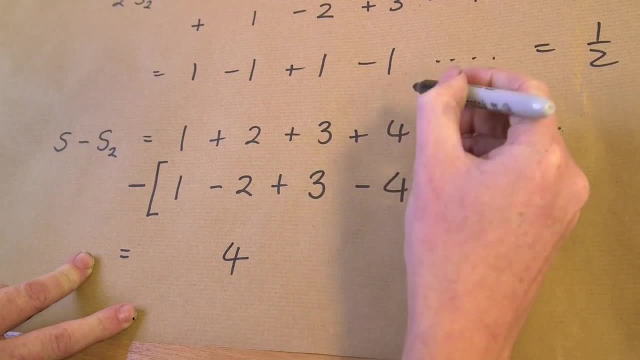 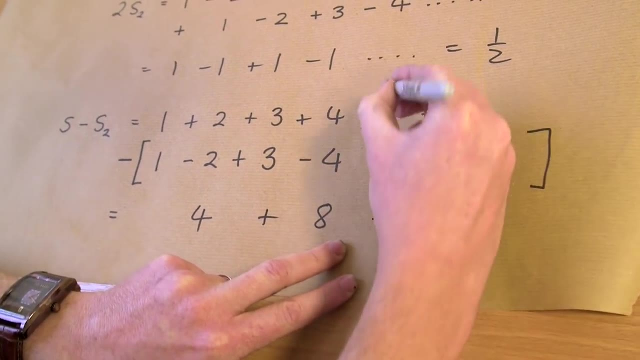 OK, 3 minus 3,, 0.. 4 minus minus 4 is 8, and so on. And the next one I'm going to get: from the 5s, I get nothing. From the 6s, I get 12, and so on. 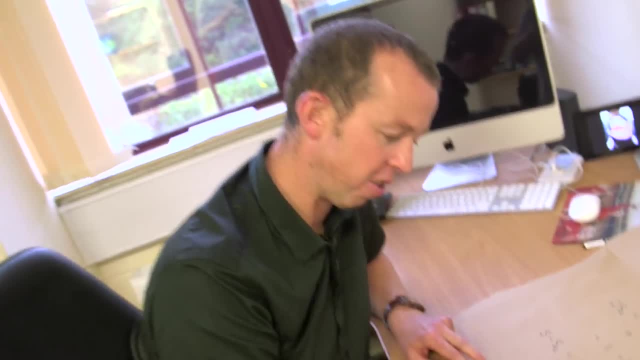 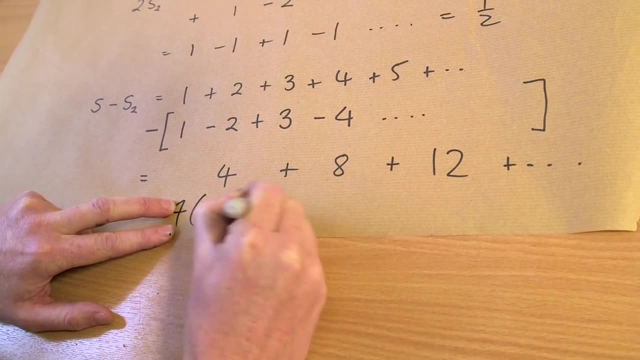 And it proceeds in that way And now you can see we're almost there now, right, Because look what I've got here. I've got 4 plus 8 plus 12.. If I take a factor of 4 out, it's 4 times 1 plus 2 plus 3.. 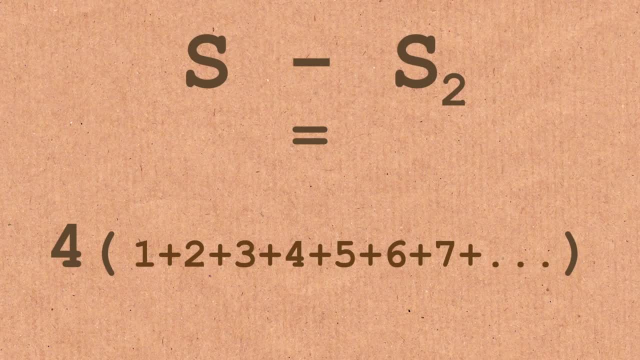 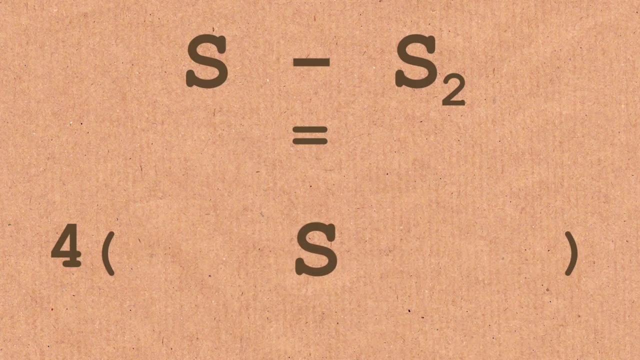 Do-do-do. OK, It's my sum that I wanted, So now I've got a formula for my- so this is just 4 times s, which is my sum. So now I just solved this equation right, Because I know what s2 is. 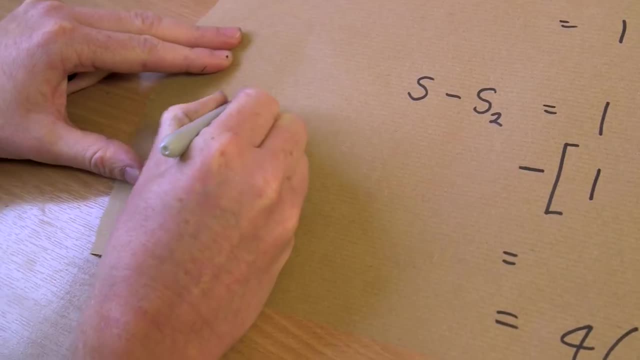 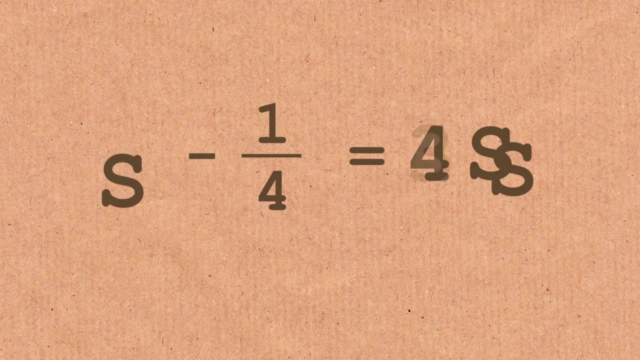 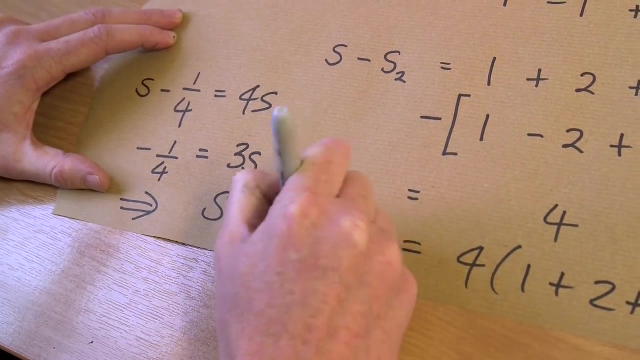 So I have now the expression s minus- because I know what s2 is. s2 is a quarter- is equal to 4s. OK, I take s from either side, so I get: minus a quarter is equal to 3s, which implies that s equals minus a 12.. 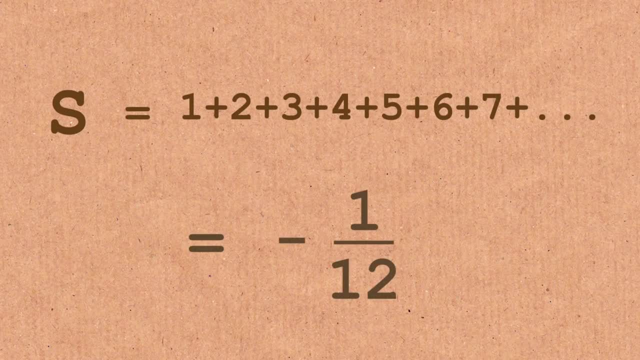 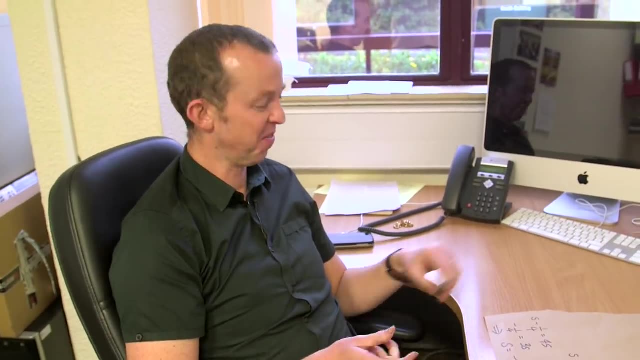 So now you've looked at it. So now do you believe me? That's amazing. I love it. It's amazing. Who'd have thought it, Tony, if I got a calculator out and wrote 1 plus 2 plus 3? 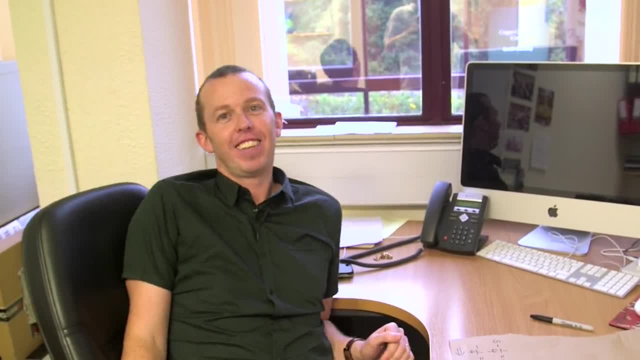 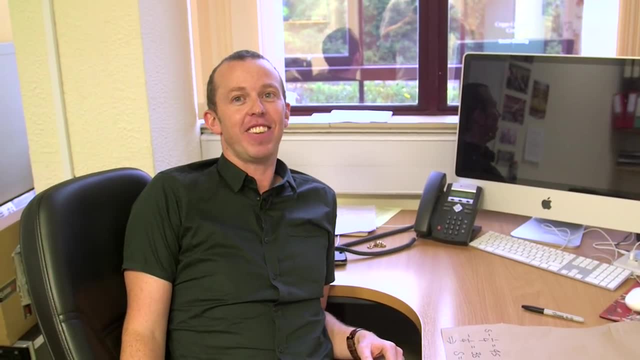 plus 4 plus 5, and I sat here until the end of everything and then pressed equals, would I get minus a 12?? I actually mean the end of everything. You can't do it to the end of everything, can you?